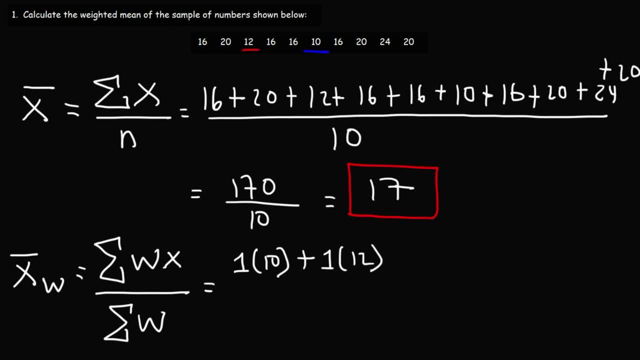 It also has a weight or frequency of 1.. Now the next number, 16, there's four of them, so it has a weight or frequency of 4, so it's going to be plus 4 times 16.. Next we have three, 20s. 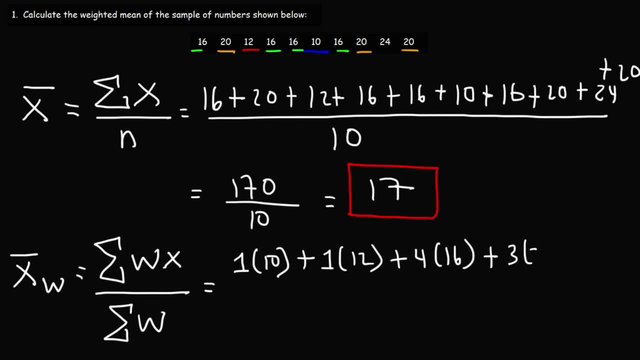 So it's going to be plus 3 times 20, and then we only have 124.. Now we need to take the sum of the weights, So that's 1 plus 1, which is 2, plus 4, that's 6, plus 9, I mean plus 3, that's 9, plus 1, that's 10.. 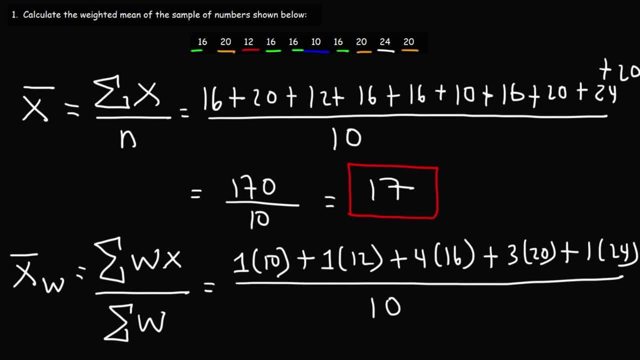 So the sum of the weights or frequencies is 10 in this example. So 1 times 3, that's 9, plus 1, that's 10.. So 1 times 3,, that's 9, plus 1, that's 10.. 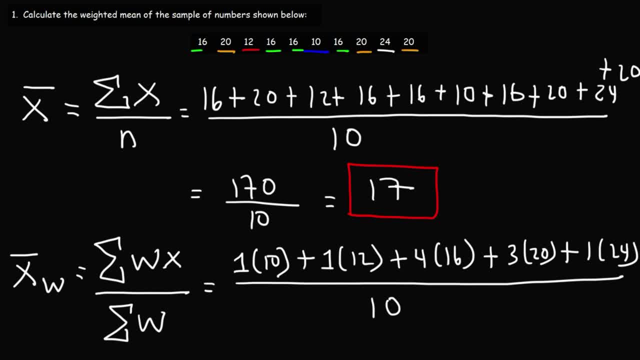 So 1 times 3, that's 9, plus 1,, that's 10.. So 1 times 10 is 10, plus 12, plus 4 times 16,, plus 3 times 20, plus 1 times 24.. 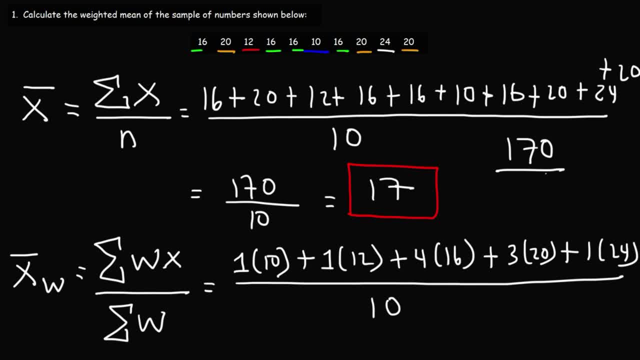 It gives us the same sum of 170.. Dividing that by 10, we're going to get the same answer of 17.. So that's how you could use this formula to calculate the weighted mean. Now let's look at another example. 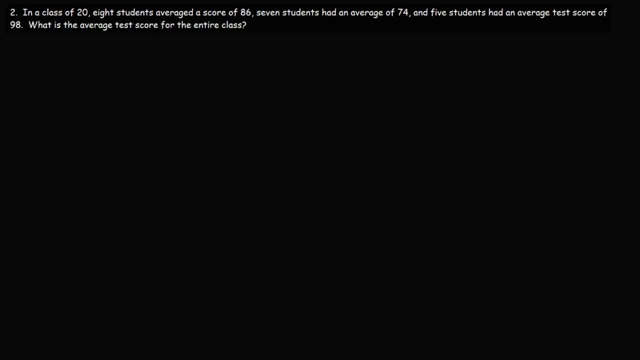 In a class of 20,, 8 students averaged a score of 86.. 7 students had an average of 74, and 5 students had an average test score of 98.. What is the average test score for the entire class? 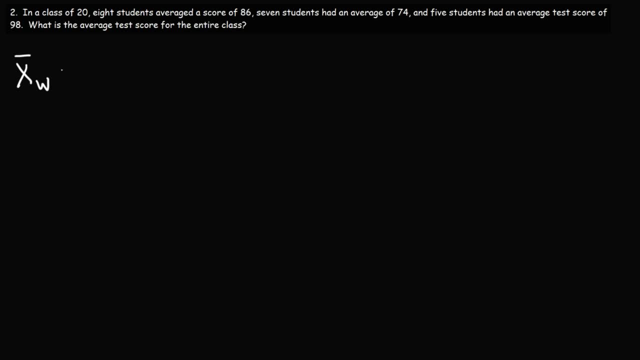 We're going to use the same formula to calculate the weighted mean, So it's going to be the sum of all the weights times each data in our sample Divided by the sum of all the weights. So first we have a weight of 8 students and an average score of 86. 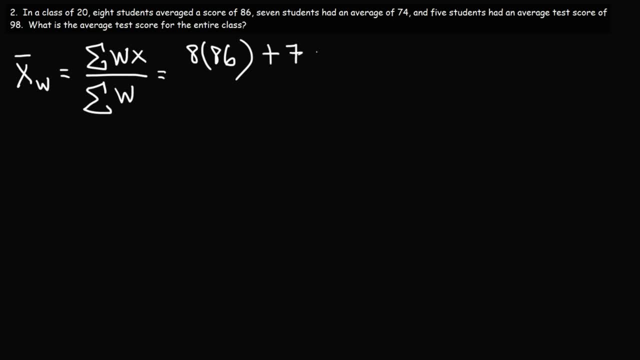 Next we have 7 students, so that's the frequency or the weight, And the average for that is 74. And then we have 5 students with an average test score of 98. Now we need to divide it by the sum of the weights. 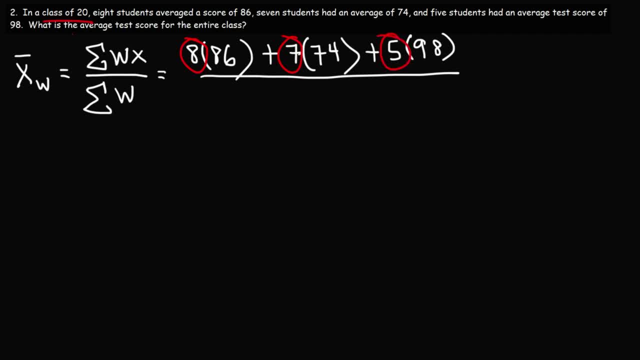 So 8 plus 7 is 7.. 7 is 15, plus 5 gives us the total of 20.. So let's do this one step at a time. First, let's multiply 8 by 86.. That's going to be 688.. 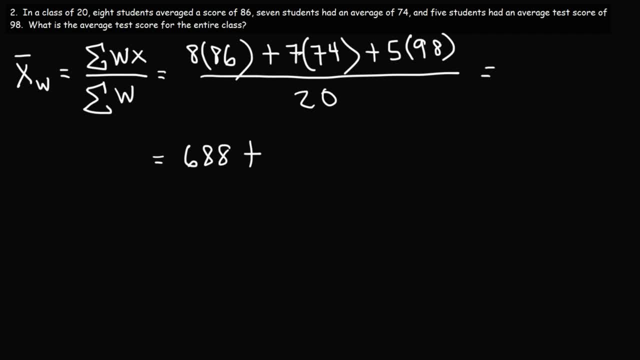 Next we have 7 times 74.. That's 518.. And then 5 times 98,, which is 490.. So taking the sum of those three numbers- 688, 518, and 490,, we have a sum of 1696.. 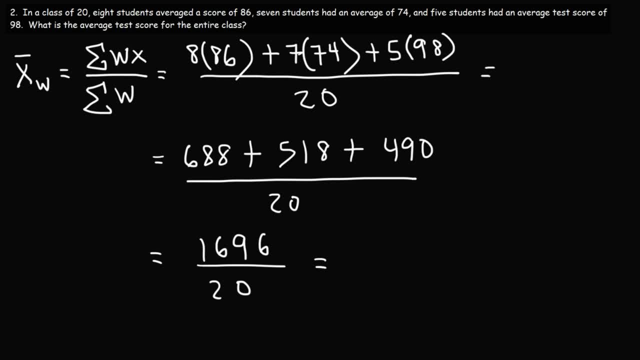 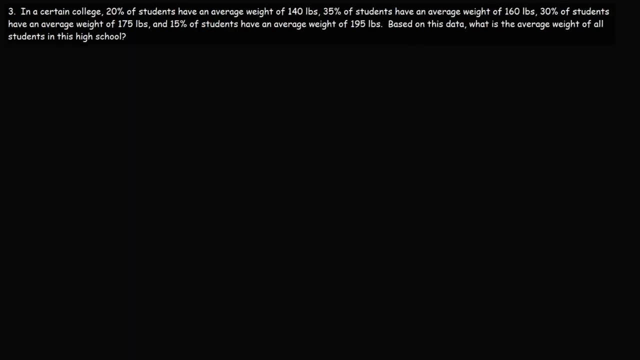 Dividing that by 20 gives us a weighted mean of 84.8.. So that is the average of all the test scores for the entire class. Now let's move on to our next problem, number 3.. In a certain college, 20% of students have an average weight of 140 pounds. 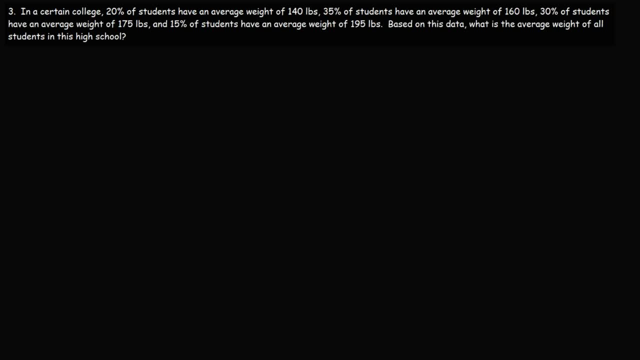 35% of students have an average weight of 160 pounds, 30% of students have an average weight of 175 pounds And 15% of students have an average weight of 195 pounds. All right, so that's a lot of information. 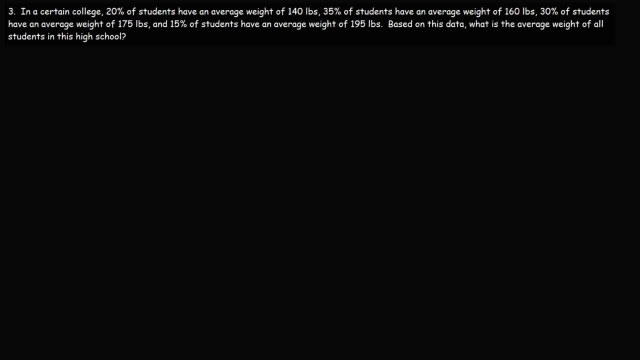 But based on this data, what is the average weight of all students In this high school? So, based on the last two previous problems, you know how to do this one. Feel free to pause the video and try it if you want to. 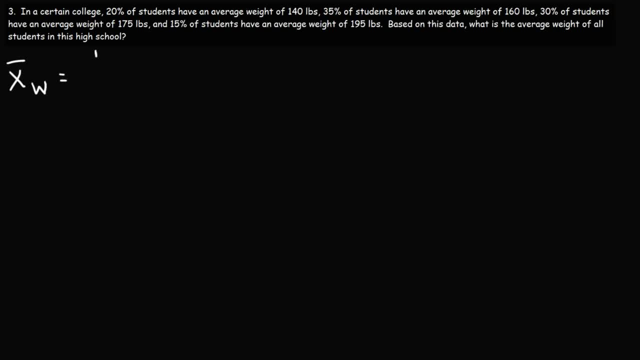 So we're going to follow the same process. We're going to multiply the weight by each data in the sample, or in this case the average, And then divide it by the sum of all the weights. So we could say X would be. 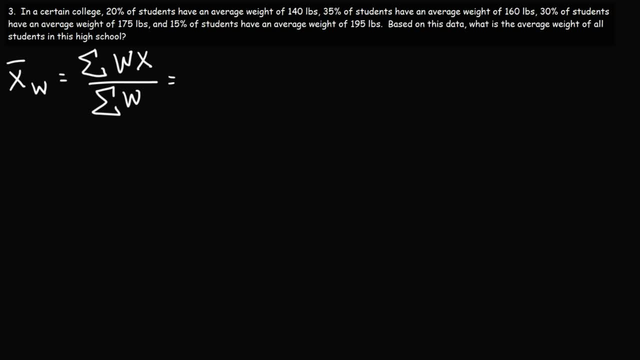 W would be the percentage that corresponds to the average weight. So for the first one, let's write this out as W1X1 plus W2X2 plus W3X3 and so forth, And then the sum of the weights will be W1 plus W2 plus W3 plus W4.. 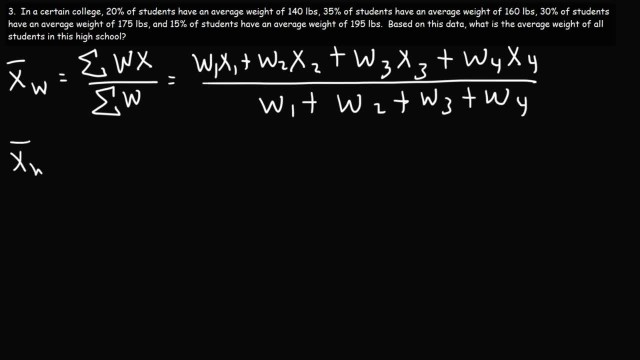 If that makes it easier. So for the first part we have 20% of students with an average weight of 140 pounds. The 20% will be the weight, X1 will be the 140 pounds, So we can write W1 as a percentage 20%. 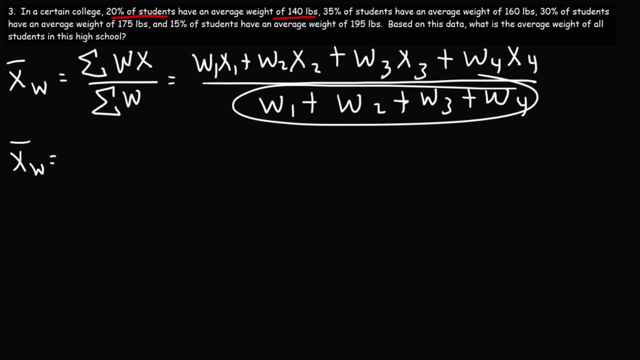 And so the total would be 100%. Or we can write that as a decimal, 0.20,, where the total would be 1.. I prefer to use The decimal version of the percentage, So W1 is going to be 0.20.. 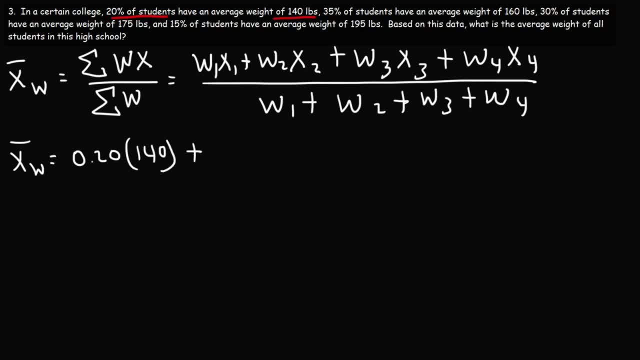 X1 is 140.. Now let's move on to the second data in our- Let me say that again- The second data point in our sample. So W2 is 35%, X2 is going to be 160.. So this is 0.35 times 160.. 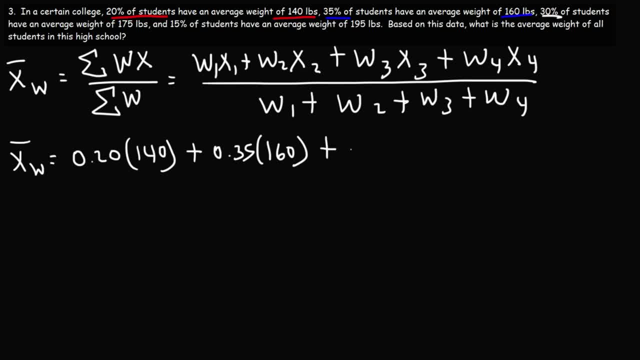 Now W3. W3. That's going to be 30% or 0.30. And X3 is 175.. Next we have W4, which is 0.15 times X4. That's 195.. So if we were to add 0.20 plus 0.35, that's 0.55. so far. 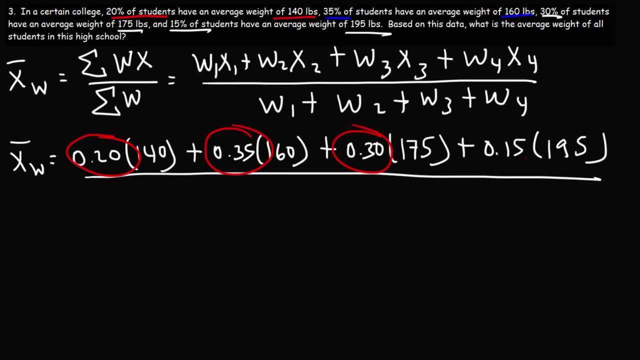 And then plus 0.3, that's 0.85.. Plus 0.15, that's going to give us 1 or 100%. So the sum of all four weights is 1.. So now let's plug in the numbers and get the answer for this problem. 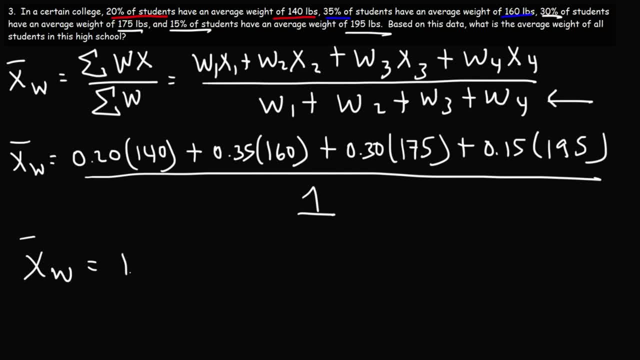 So the weighted average for this example problem Is going to be 160.. And so that's it for this problem. That's how you can calculate the average weight of all students in this high school. Now let's move on to our next example problem. 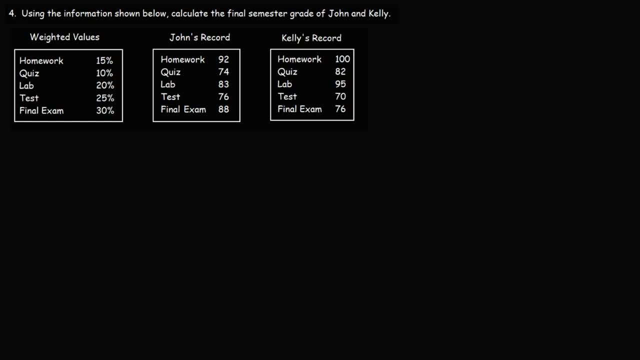 Number four, Using the information shown below, calculate the final semester grade of John and Kelly. So we're going to use the same formula to do so. It's going to be the sum of the product of the weight and the data point in our sample, X1.. 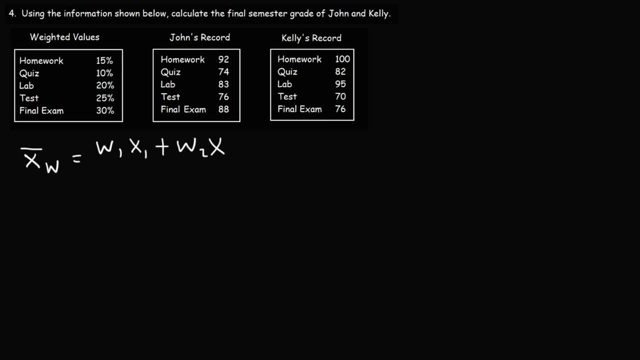 So it's going to be W1X1 plus W2X2.. And since we have five things we're dealing with, we're going to go up to W5X5.. And then we're going to divide it by the sum of all of the weights. 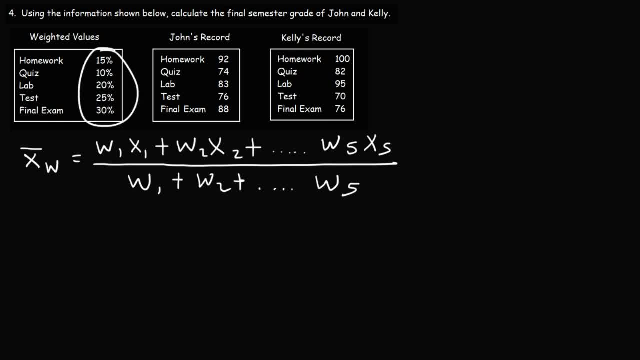 Since the weights are given as percentage values, the sum is going to be 100% or one as a decimal number. So let's start by calculating the weighted mean for John. So W1 is going to be the 15%, So that's 0.15.. 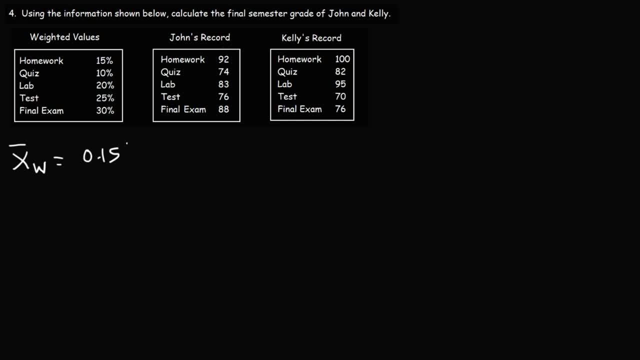 And the homework score for John is 92. So that's going to be X1.. Next we have W2.. So that's going to be The weighted percentage for the quiz, which is 10% times the quiz score of 74.. 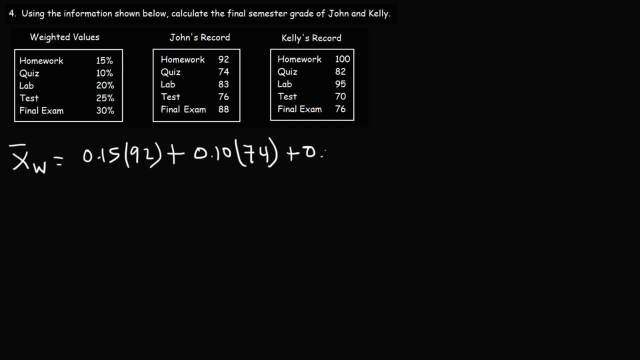 And then we're just going to repeat the process. So for the lab it's 0.20. And the score for that is 83.. Next we have the tests which has a weighted value of 25% or 0.25,. 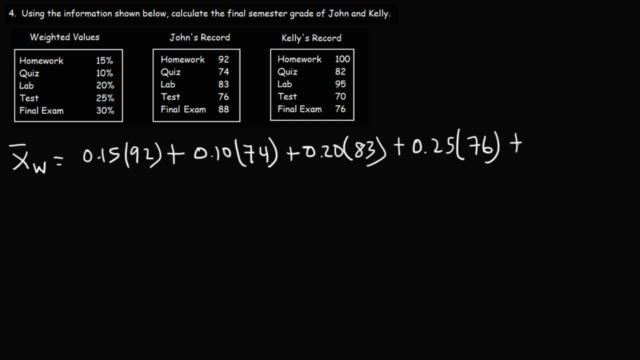 times the score of 76.. And then the final exam is, which has a weighted 30% times the score of 88. So now we're going to divide by the sum of all the weights 0.15 plus 0.10, that's 0.25. 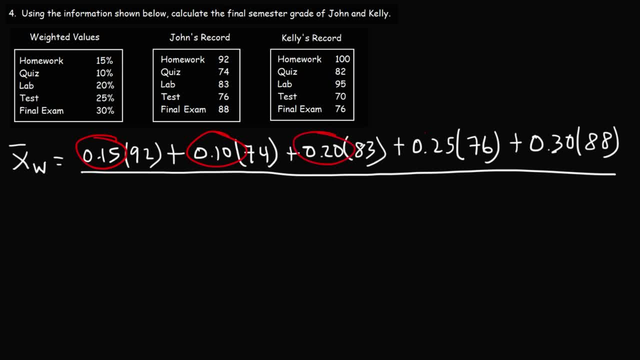 Plus 0.20, that's 0.45.. Plus 0.25, that's 0.7.. Plus 0.3, that's 1.. So you really don't need to put the 1, since it's not going to change your answer. 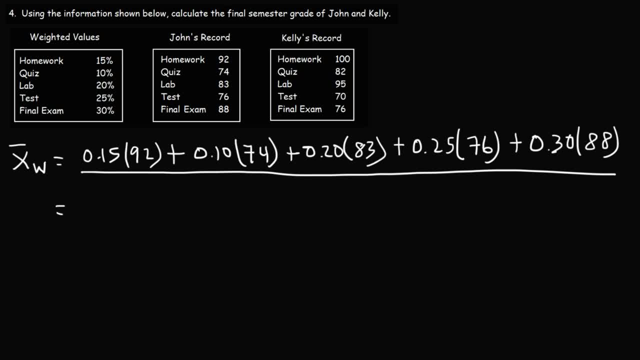 So this comes out to be a final exam score, or rather a final semester grade of 83.2 for John. Now let's do the same thing for Kelly. Feel free to pause the video and try it yourself. So the homework percentage will still be 0.15,. 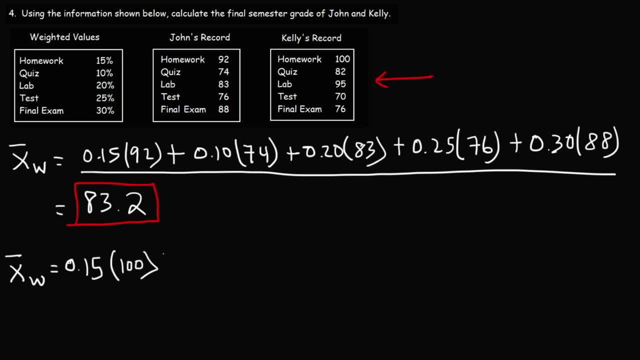 but Kelly's homework score is 100, so that's different. And then for the quiz it's going to be 10% or 0.10.. Her quiz score is 82, and then it's going to be plus 0.20,. 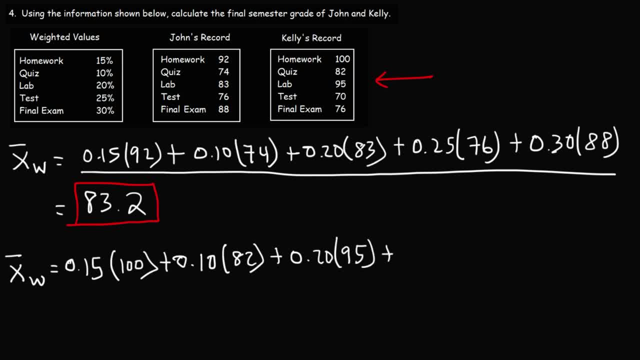 times her lab score of 95,, plus 0.25, times her test score of 70, and then plus 0.30, times her final exam score of 76. And we don't need to divide it by 1,. 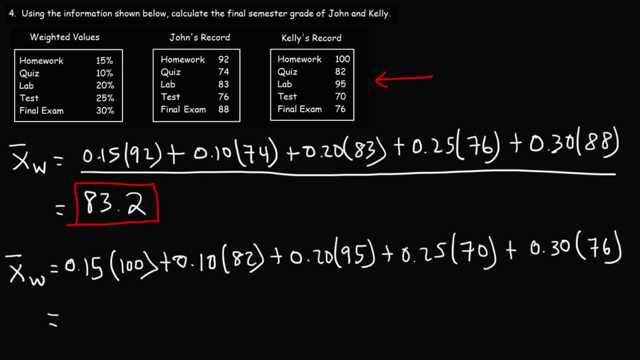 so we can just leave it like that. So all we got to do is just plug these numbers into the calculator and see what the final result is. So the final answer that I got is 82.5.. 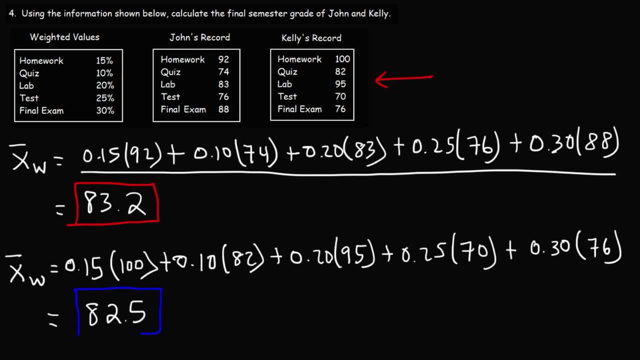 So in this example, John has a higher final semester grade than Kelly. Now let's talk about why that's the case. If you notice, his test and final exam score is significantly higher than Kelly's, And also these two categories have a higher weight. 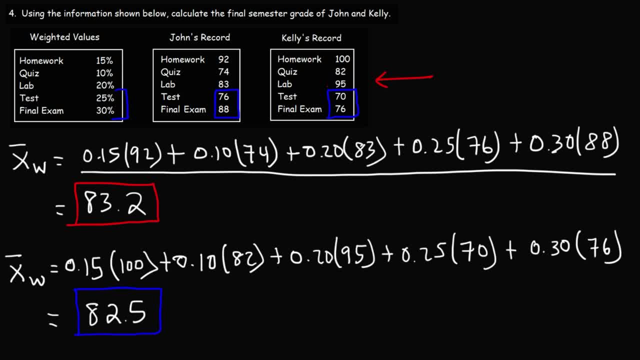 than the other three categories, even though Kelly did better on her homework lab and quiz score than John. The total weight of those three categories is 45%, compared to the weight of the test and the final exam categories, which is 55%. 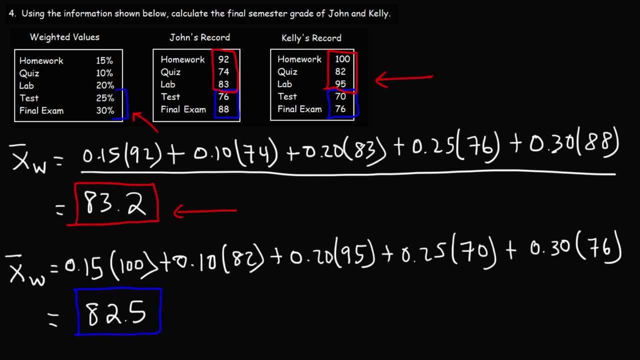 So because he did better in areas that weighted more or that carried more weight, his score was slightly higher than Kelly's score, And so that's it for this problem. Now you know how to calculate your final semester grade, if you know the weighted percentage values. 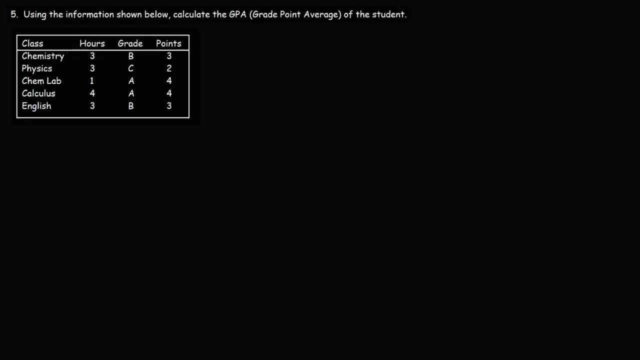 for each of these categories, Number five, Using the information shown below, calculate the GPA or the grade point average of the student. So we're going to use the same formula that we've been using: W1X1 plus W2X2. 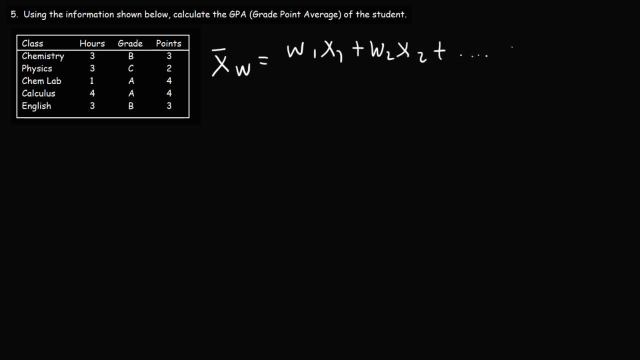 in this case, all the way to W5X5 divided by the sum of the weights. Now we need to determine what's X and what's the weight. We want to calculate the average grade point or the grade point average, not the average hours. 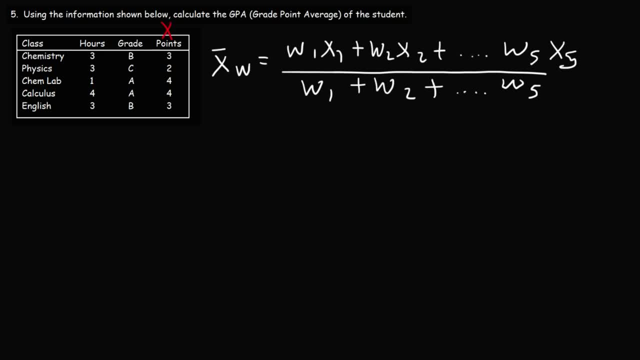 So we want the average of the points. So the points will be X, the weight will be the hours, W1 will correspond to chemistry. that's going to be the hours to chemistry. that's three. X1 will be the point score. 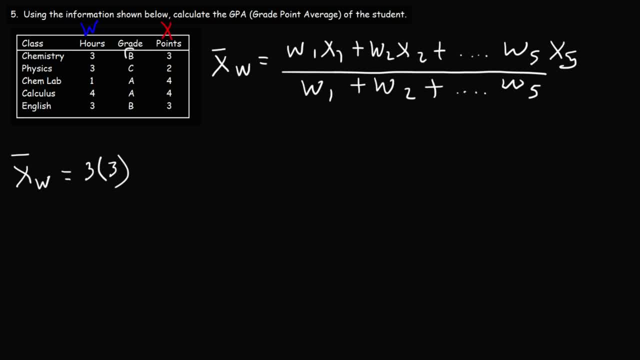 for chemistry, which is three. So anytime you have a, B, that corresponds to a, three, An A corresponds to four points, A, C corresponds to two, And the credit hours of the course is just dependent on what type of course you're dealing with. 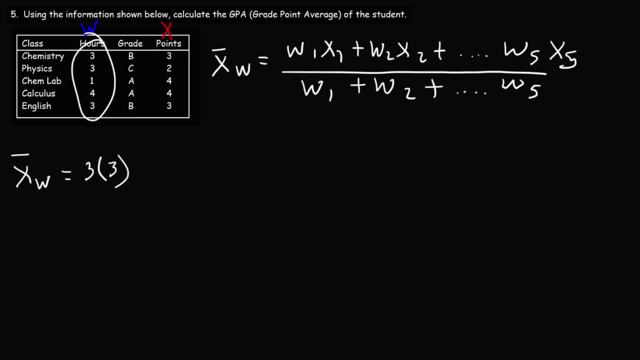 For a lab. it's a one credit hour course. in college- at least the college that I went to- A typical chemistry course could be three credits, Some may even be four, But let's go ahead and finish this problem. So W2 is going to correspond to physics. 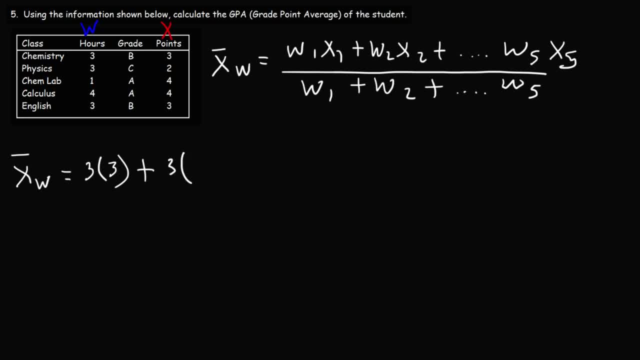 that's the hour. credit for physics and the score for that: X2, the point score was two. Now for W3, it's going to be one and the point score for that is four. And then for W4, calculus. 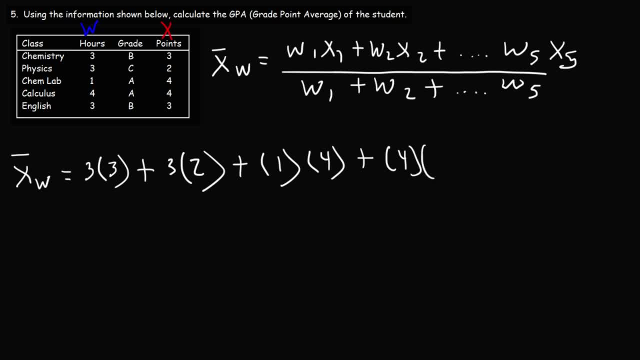 it has four credit hours. he got an A in the class, so that's four points, And then W5, it's three credit hours for English times. three points for a- B. Now we need to add up all of the credit hours. 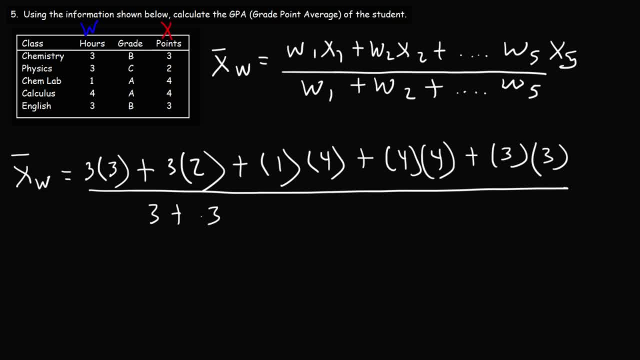 So it's going to be three plus three plus one plus four plus three, So that's W1, all the way to W5.. So now we can do the math. Three times three is nine, three times two is six. 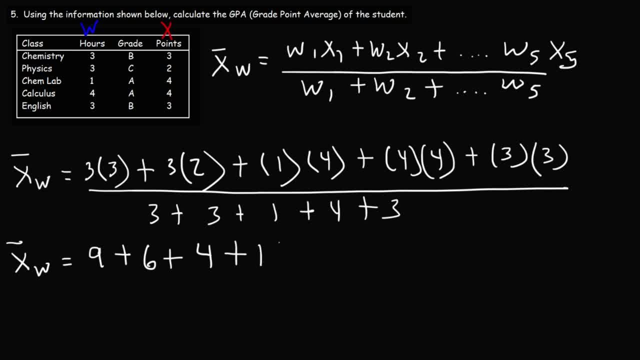 four times one is four, four times four is sixteen, three times three is nine. And then we have three plus three, which is six, seven, eleven, fourteen. So we have a total of fourteen credit hours, So nine plus six. 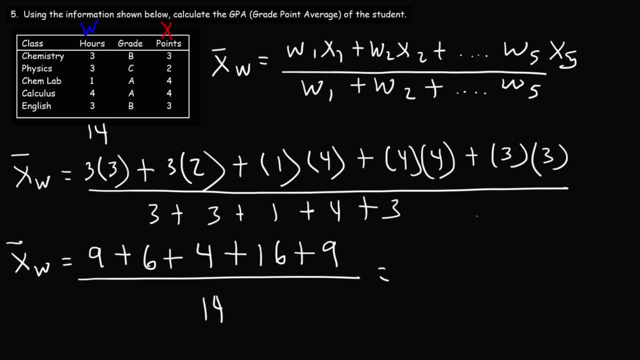 plus four plus sixteen plus nine, that's going to be forty-four divided by fourteen. That gives this student a grade point average of three point one four, which is close to a- B. So that's how you can calculate the grade point average. 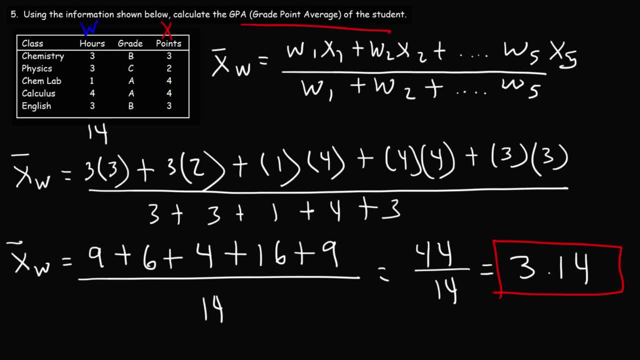 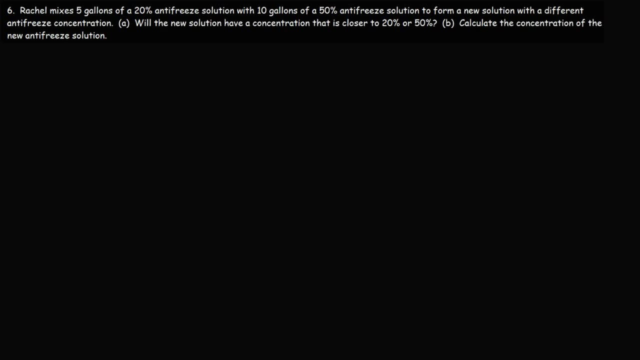 of a student, if you know the credit hours of the courses that he has and if you know the letter grade for each of those courses. Number six: Rachel mixes five gallons of a twenty percent anti-free solution with ten gallons of a fifty percent. 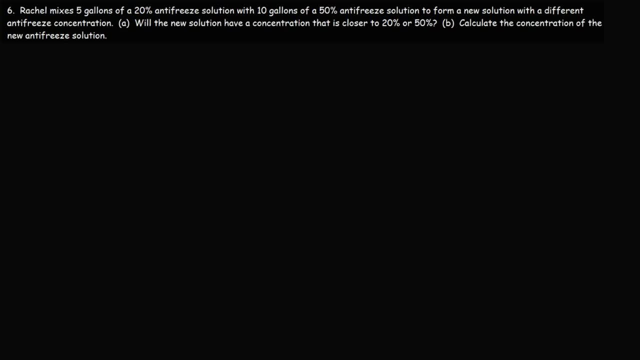 anti-free solution to form a new solution with a different anti-freeze concentration? Will the new solution have a concentration that is closer to twenty percent or fifty percent? What would you say? So let's say we have solution one and solution two. 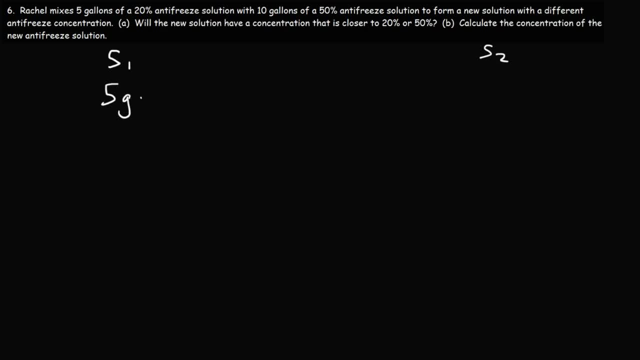 So solution one has a volume of five gallons And solution two has a volume of ten gallons. Now the concentration of solution one is twenty percent. The concentration of solution two is fifty percent. We want to calculate the concentration of the combined solution. 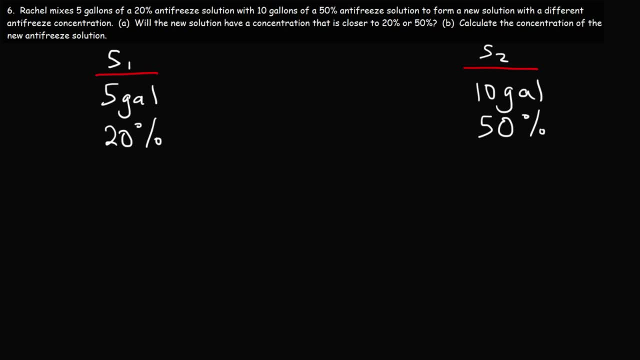 So, based on that, what's a W and what's X? X is what we want to find the average of. So this is X one and that's X two. The weight in this case will be the volume. 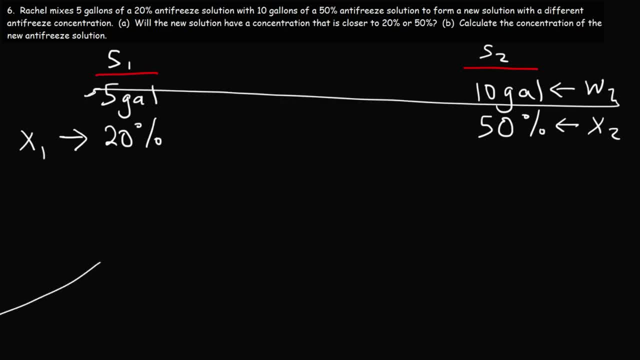 That will be W two. Whoa, what just happened there. Sometimes this computer can act up, It has issues, But this is what we have for this problem so far. Now the combined solution, or let's call it solution three. 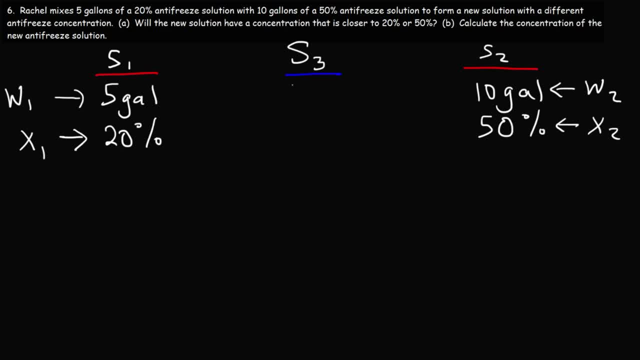 it's going to have a total volume of fifteen gallons, Because once you mix a five gallon solution with a ten gallon solution, we're going to get a fifteen gallon solution. What we need to calculate is the average or the weighted concentration of that solution. 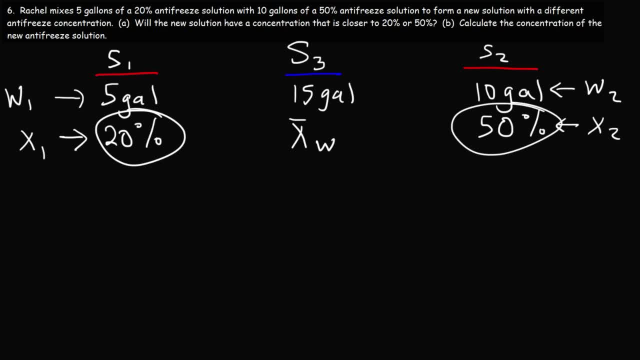 Now, if you were to average twenty and fifty, assuming they have equal weights, the midpoint of twenty and fifty is thirty-five. Now, because the weights are not equal, we know the answer won't be thirty-five, But is the answer closer to twenty percent? 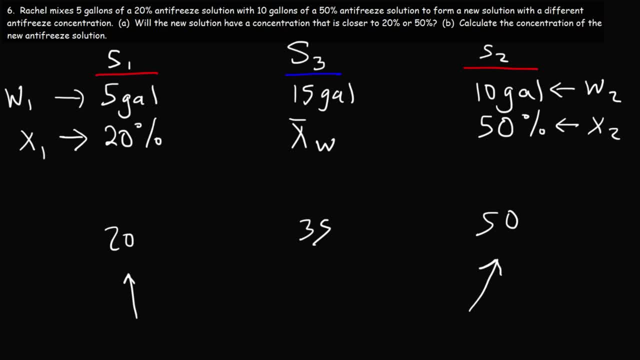 or is it closer to fifty percent? What would you say? So take a minute and think about that. Will the average concentration, I mean the new anti-freeze concentration, will it be between twenty and thirty-five, or thirty-five and fifty? 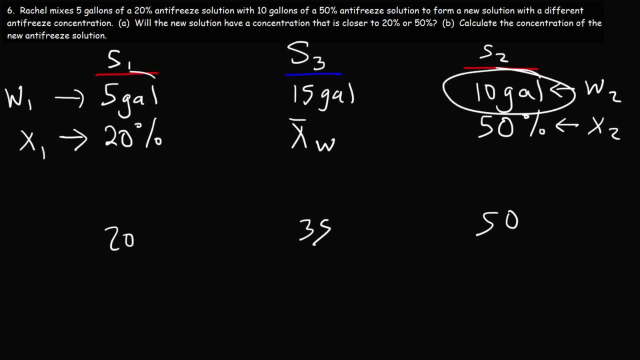 Now notice that solution two carries more weight than solution one. Therefore, the combined solution should have a concentration somewhere between thirty-five and fifty, And so I'm going to write that It should be somewhere between thirty-five and fifty percent, because solution two carries. 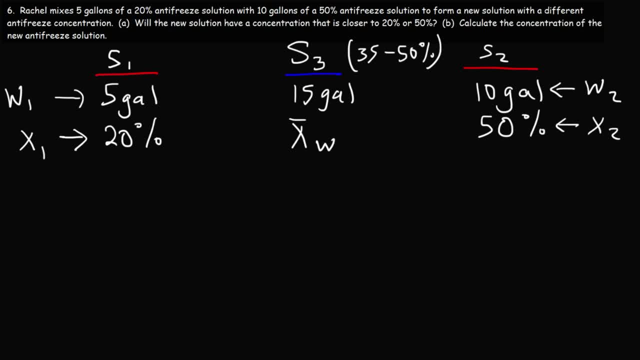 more weight than solution one, So it's going to be closer in concentration to solution two. So now let's calculate the weighted average or the new concentration of the anti-freeze solution. So it's going to be the sum of the weights times. 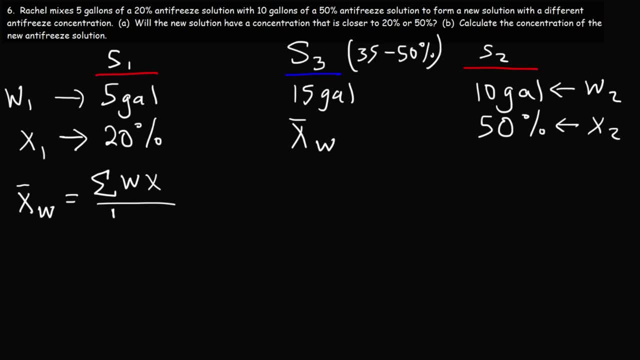 in this case the concentrations divided by the sum of the weights. So it's going to be W1X1 plus W2X2 divided by W1 plus W2.. So W1 is five gallons And X1, the concentration. 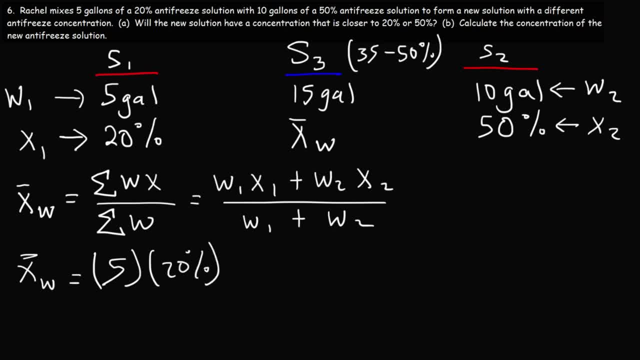 is twenty percent. This time I'm going to leave it in percentage. I'm not going to convert it to point twenty, because I want my final answer to be in percent. Now, W2 is ten gallons and X2 is fifty percent. 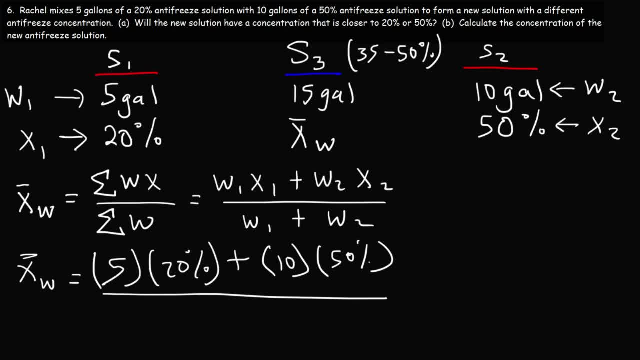 Now we're not taking the sum of the percentages, We want to average the percentages. We need to take the sum of these two numbers: W1 plus W2, is five plus ten. So we have five times twenty, which is a hundred. 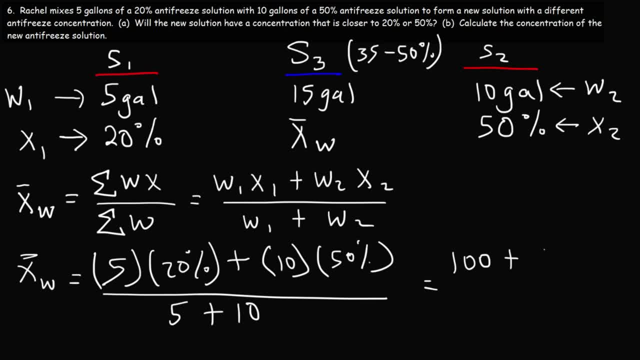 and then plus ten times fifty, That's going to be five hundred divided by fifteen. So that's six hundred divided by fifteen, and that's going to give us an average weighted concentration of forty percent. So this is the answer. By the way, 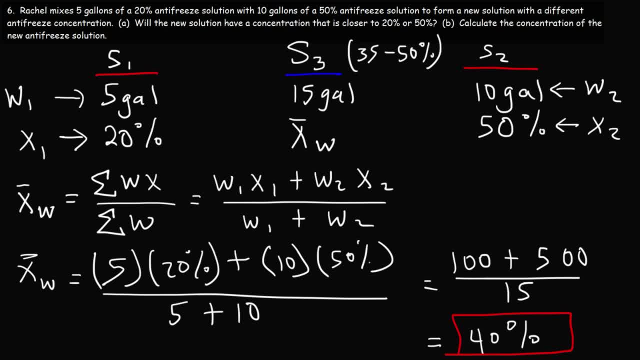 for those of you who like to focus on units, this is in gallons, so that's percent, That's gallons percent. When you add these two, that's going to be in gallons, So the unit gallons will cancel, leaving behind the unit percent. 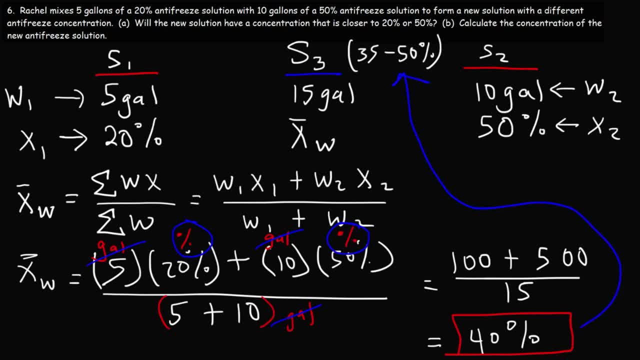 Now, as we can see, our answer is well within this range. It's between thirty-five and fifty percent. So solution three has a concentration that is closer to solution two, because solution two carries more weight than solution one, And that's how weighted averages work. So that's it for this video. Thanks again for watching. 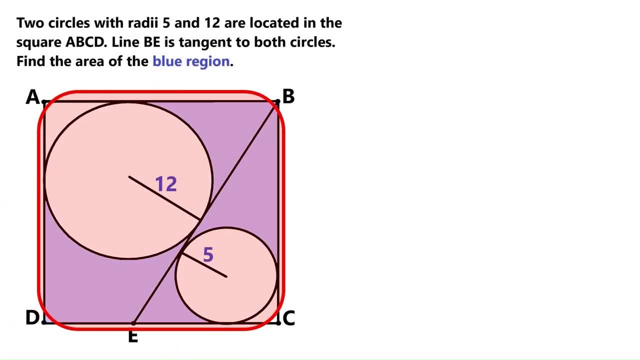 In this super cool geometry problem. we've got this square ABCD and these two circles are inside the square. This big circle's radius is 12 and this small circle's radius is 5. The circles don't touch, but we've got this line, segment EB, that is tangent to both circles.